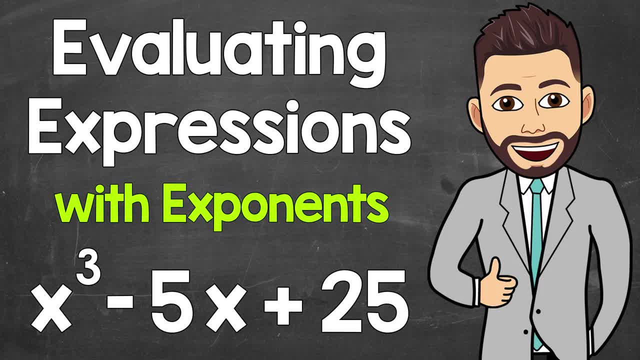 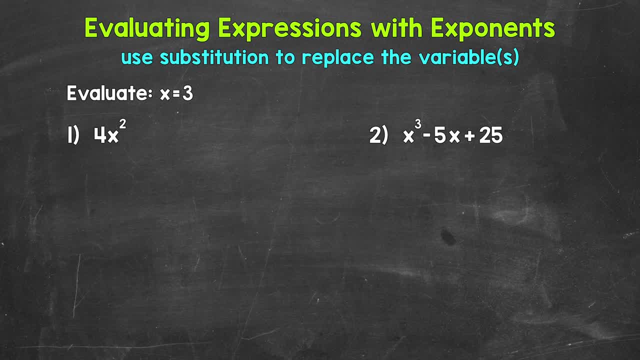 Welcome to Math with Mr J. In this video I'm going to cover how to evaluate expressions with exponents. Now, when we evaluate an expression, we find the value of the expression, so what it equals once we work through it. For our examples, we are going to evaluate the expressions when x equals 3.. 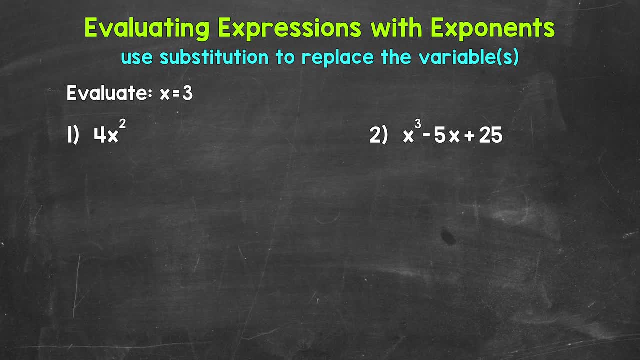 Let's jump into number 1, where we have 4x squared, so 4 times x squared. Remember that exponent tells us that we are multiplying the base, which is x in number 1, by itself, a certain number of times. 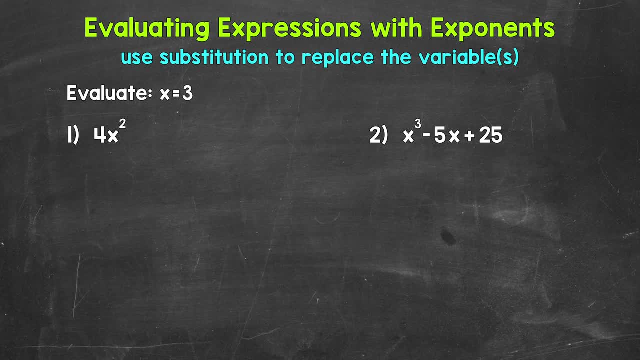 The exponent tells us how many times. For example- let me come to the side here- x squared means x times x. We expand that base out however many times the exponent tells us and we multiply Now that we know what that exponent means. 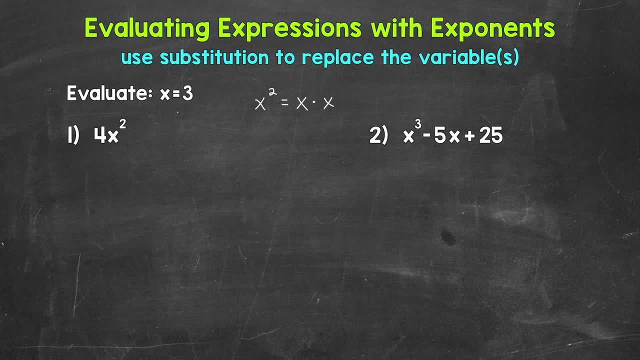 the first thing that we need to do as far as evaluating this expression, we need to replace or plug in the given value for the variable. This is called substitution, So let's plug in 3 for x and rewrite this expression, So we have 4.. 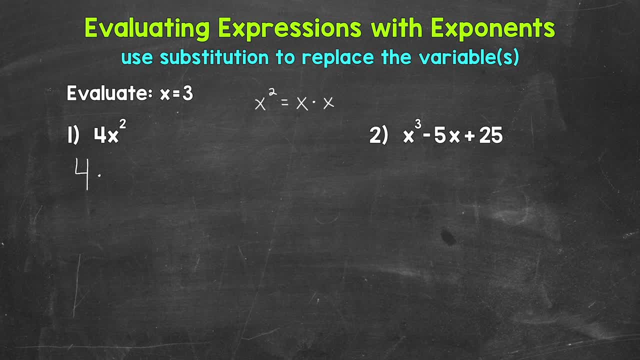 4 times x squared, Plug in 3 for x and then that exponent of 2.. Now we can evaluate. So let's figure out what this equals. Exponents come before multiplication, as far as the order of operations go, So let's start with 3 squared. 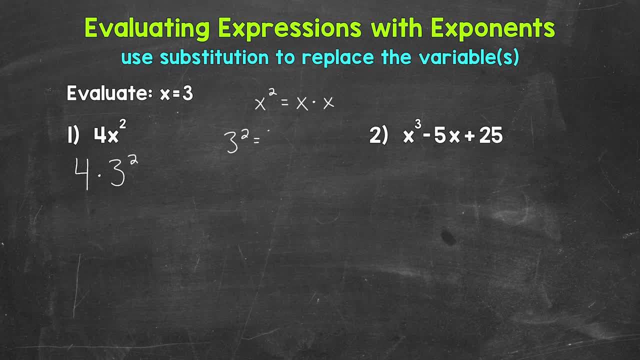 3 squared. well, that means 3 times 3.. 3 times 3. 3 equals 9.. So 3 squared equals 9.. Bring down everything we did not use and we end with multiplication. So 4 times 9.. 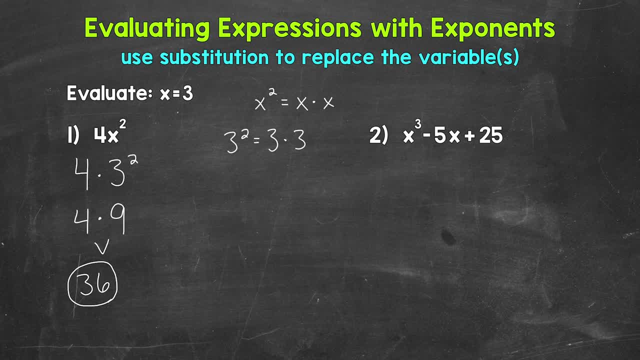 That equals 36.. The value of this expression is 36 when x equals 3.. Let's move on to number 2, where we have x cubed minus 5x plus 25.. Now, x cubed, that means x times x times x. 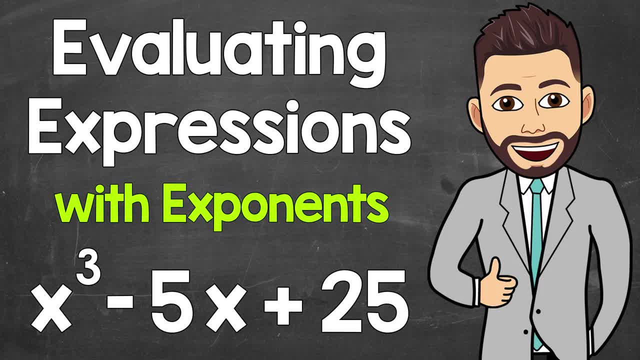 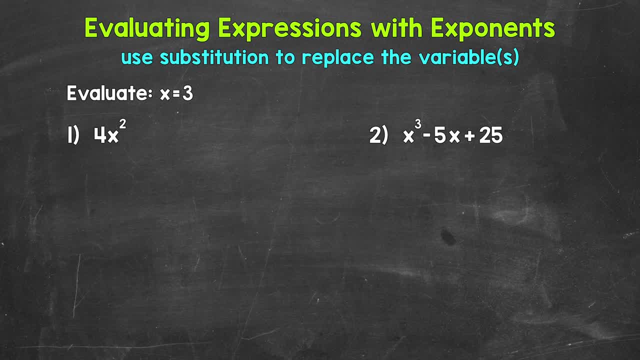 Welcome to Math with Mr J. In this video I'm going to cover how to evaluate expressions with exponents. Now, when we evaluate an expression, we find the value of the expression, so what it equals once we work through it. For our examples, we are going to evaluate the expressions when x equals 3.. 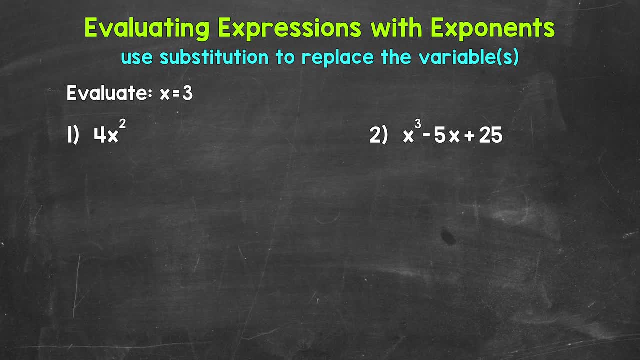 Let's jump into number 1, where we have 4x squared, so 4 times x squared. Remember that exponent tells us that we are multiplying the base, which is x in number 1, by itself, a certain number of times. 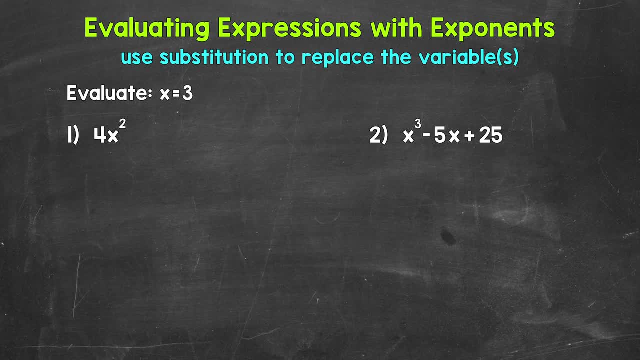 The exponent tells us how many times. For example- let me come to the side here- x squared means x times x. We expand that base out however many times the exponent tells us and we multiply Now that we know what that exponent means. 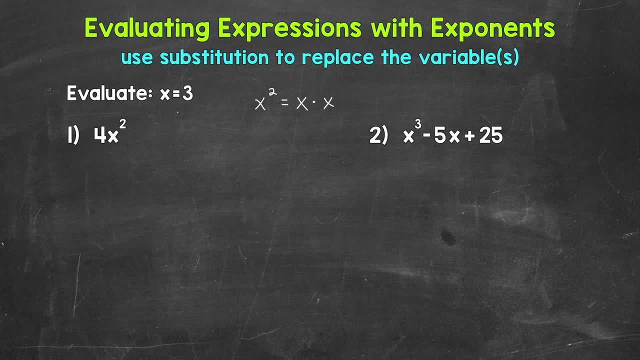 the first thing that we need to do as far as evaluating this expression, we need to replace or plug in the given value for the variable. This is called substitution, So let's plug in 3 for x and rewrite this expression, So we have 4.. 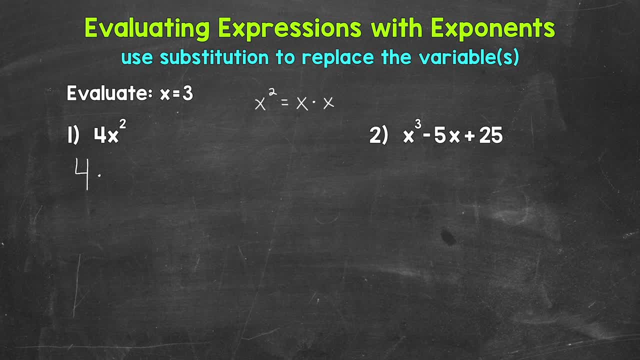 4 times x squared, Plug in 3 for x and then that exponent of 2.. Now we can evaluate. So let's figure out what this equals. Exponents come before multiplication, as far as the order of operations go, So let's start with 3 squared. 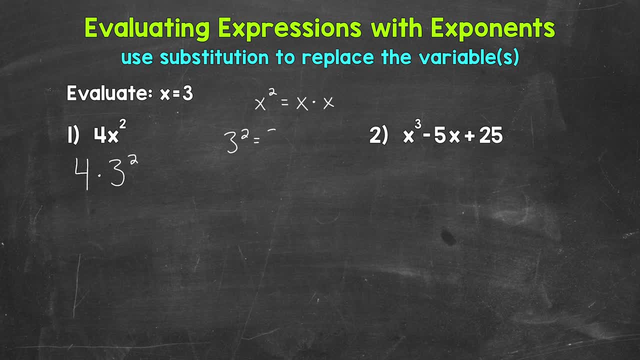 3 squared, well, that means 3 times 3.. 3 times 3. 3 equals 9.. So 3 squared equals 9.. Bring down everything we did not use and we end with multiplication. So 4 times 9, that equals 36.. 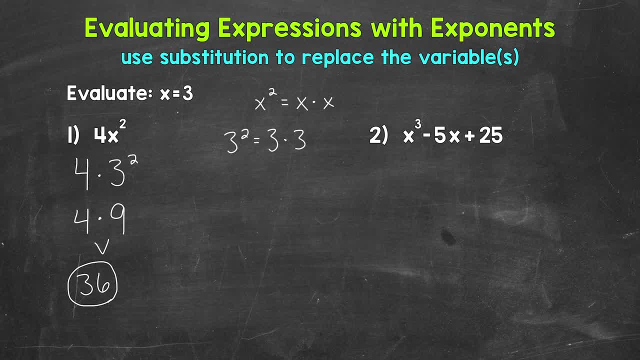 The value of this expression is 36 when x equals 3.. Let's move on to number 2, where we have x cubed minus 5x plus 25.. Now, x cubed, that means x times x times x. 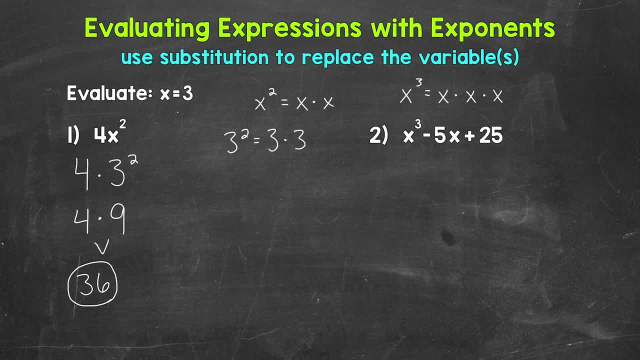 Let's plug in and evaluate: So x equals 3.. So we have 3 cubed minus 5 times x, So 5 times 3 plus 25.. Now in this expression we have an exponent subtraction, multiplication and addition. 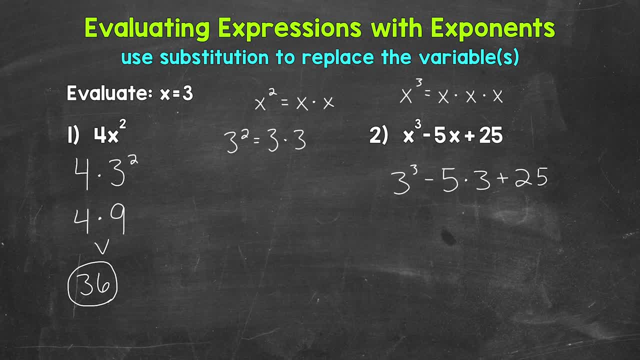 So let's work through the order of operations. Do we have any parentheses? No, Do we have any exponents? Yes, So let's start there. We have 3 cubed, So let's come to the side here. 3 cubed, well, that means 3 times 3 times 3.. 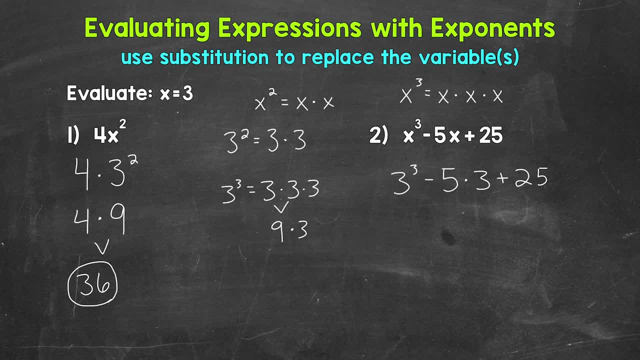 3 times 3 is 9 times 3 is 27.. So 3 times 3 times 3.. 5 times 3 equals 27,. or 3 cubed equals 27.. Let's bring down everything we did not use. 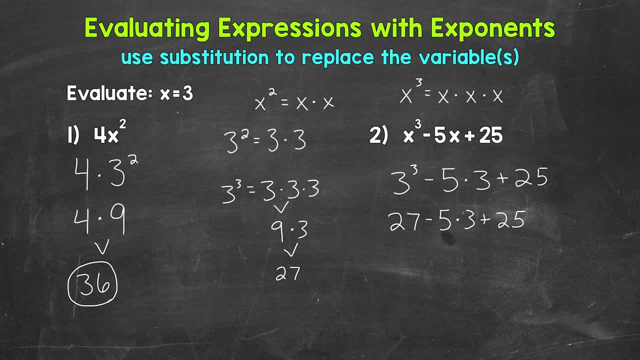 Now we have subtraction, multiplication and addition. Multiplication comes before addition and subtraction, So let's do 5 times 3 next, which equals 15.. Bring down everything we did not use. 5 times 3 equals 27.. 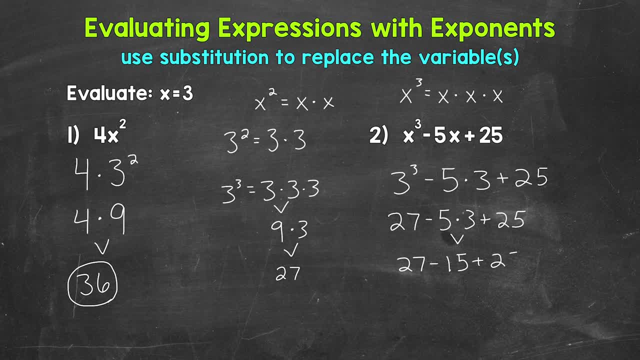 Multiplication comes before addition and subtraction. So now we have subtraction and addition, which are the same priority, so to speak. So what we can do, we can work from left to right. Subtraction comes first in this expression, So let's do 27 minus 15 next. 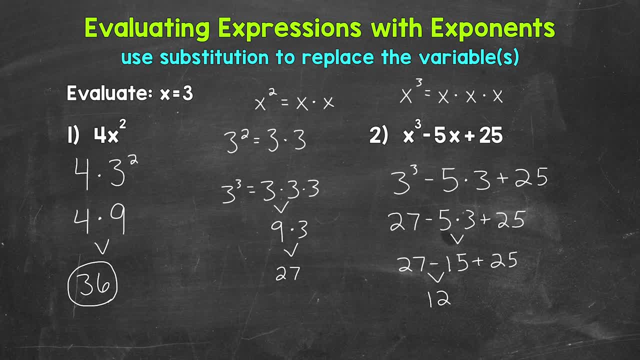 27 minus 15 equals 12.. Bring down what we did not use And we end with addition 12 plus 25, that equals 37. The value of this expression is 37 when x equals 3.. So there you have it. 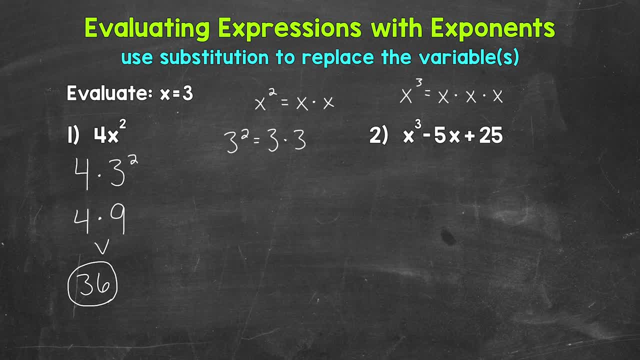 Let's plug in and evaluate: So x equals 3.. So we have 3 cubed minus 5 times x, So 5 times 3 plus 25.. Now in this expression we have an exponent, subtraction, Multiplication and addition. 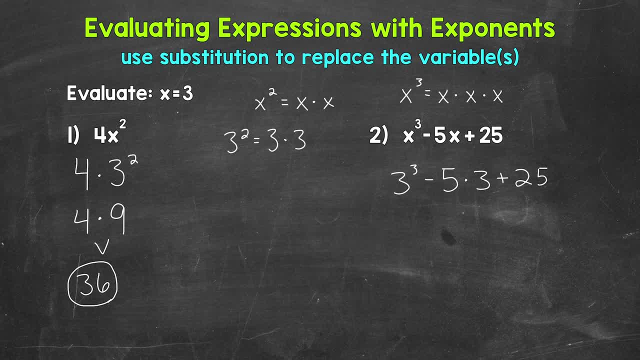 So let's work through the order of operations. Do we have any parentheses? No, Do we have any exponents? Yes, So let's start there. We have 3 cubed, So let's come to the side here. 3 cubed, well, that means 3 times 3 times 3.. 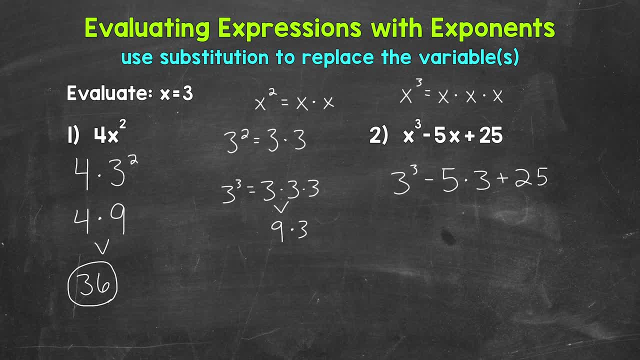 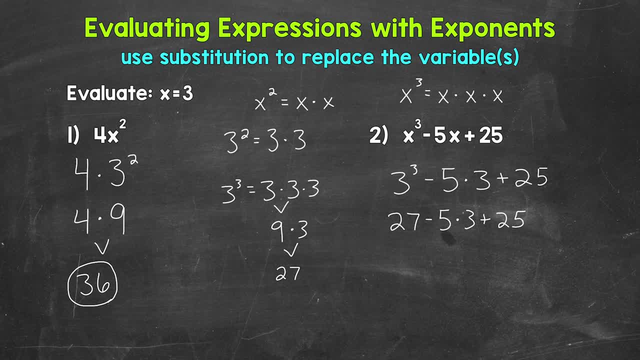 So 3 times 3 times 3 is 27.. Now we have subtraction, multiplication and addition. Multiplication comes before addition and subtraction, so let's do 5 times 3 next, which equals 15.. Bring down everything we did not use. 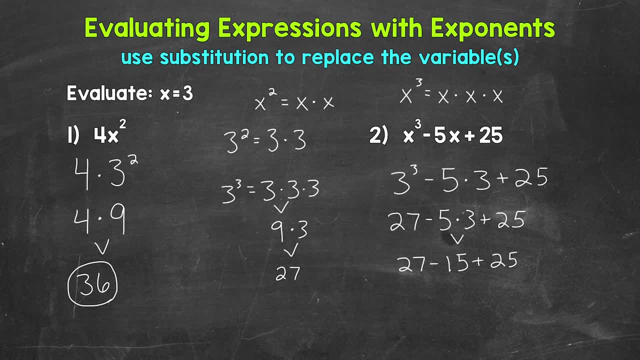 So now we have subtraction and addition, which are the same priority, so to speak. So what we can do, we can work from left to right. Subtraction comes first in this expression, so let's do 27 minus 15 next.